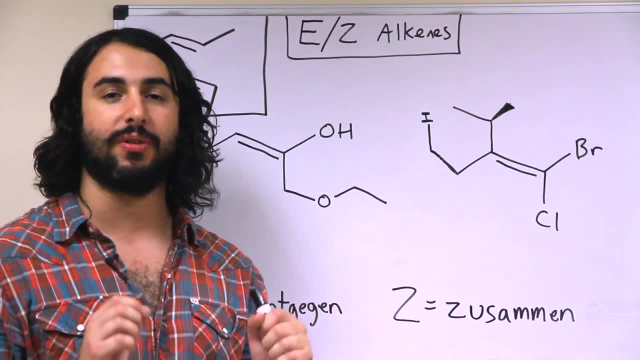 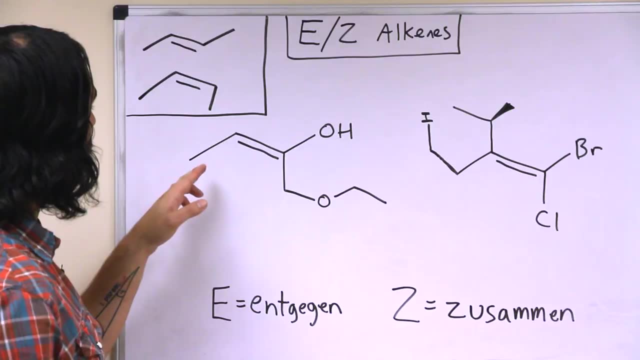 we're going to assign the priority of one group over the other by going one atom at a time, So sometimes we'll only have to go one atom along. So basically here this carbon is attached to a carbon and the implied hydrogen. 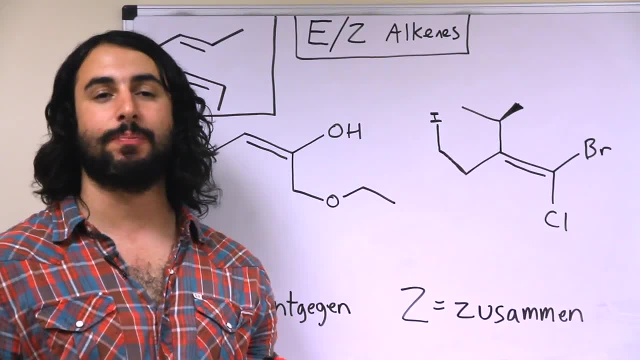 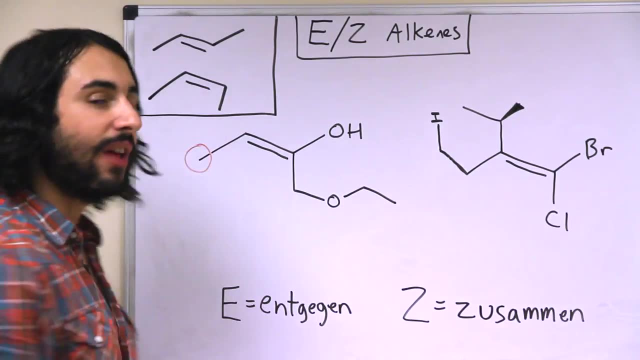 So remember that we're going by atomic mass here. So it's simply that carbon is heavier than hydrogen is the reason that this group wins. So for the left, carbon: we've decided that it's the carbon that takes priority down here. 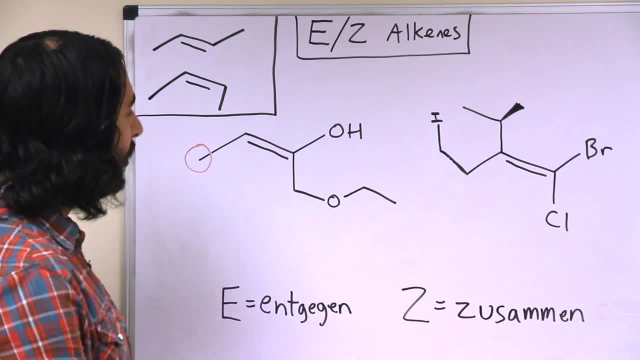 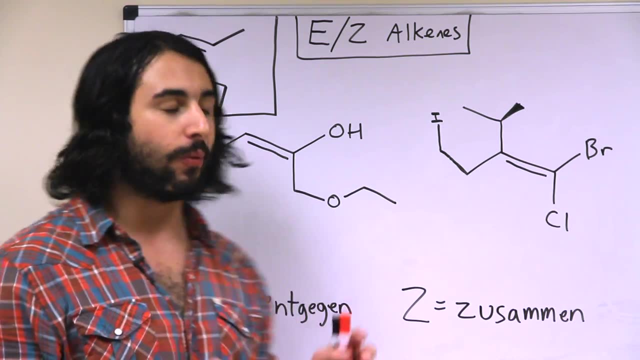 over the implied hydrogen. So now on the right side, this is where we have to recall that we must put on our blinders and go one atom at a time, Because if we didn't do that, we might look at this side and say: 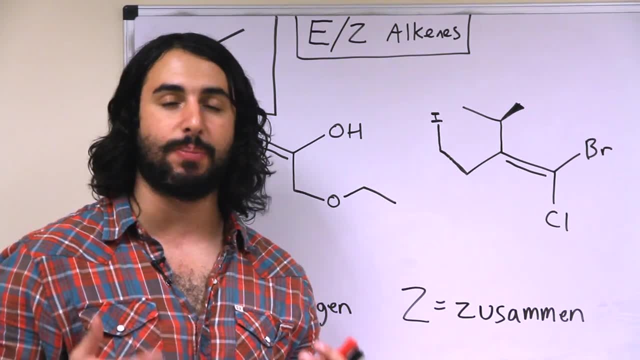 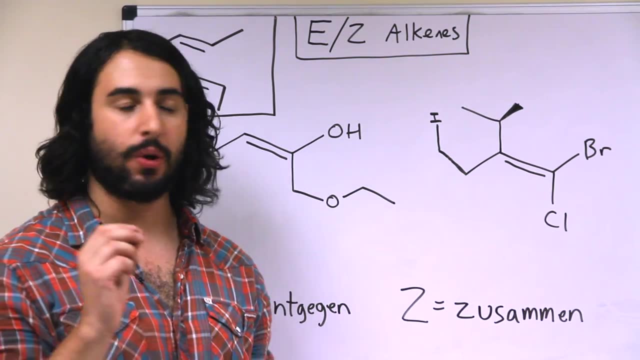 well, clearly, this group takes priority because it's bigger, it's bulkier, it's heavier, So that's going to take priority. However, that's not going to be the case because, recall, we're going one atom at a time. 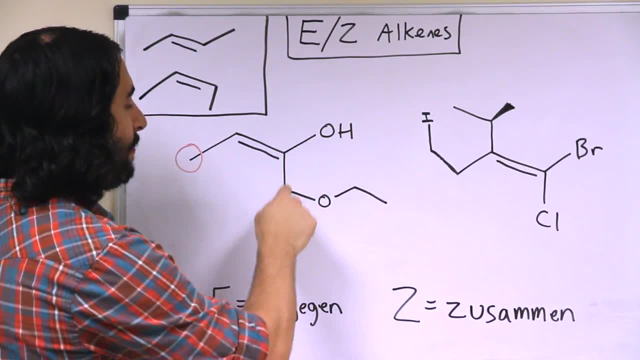 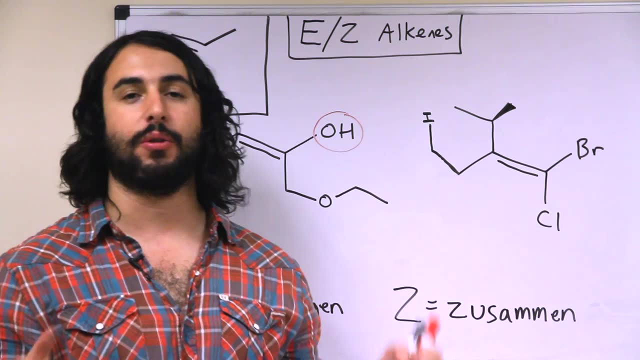 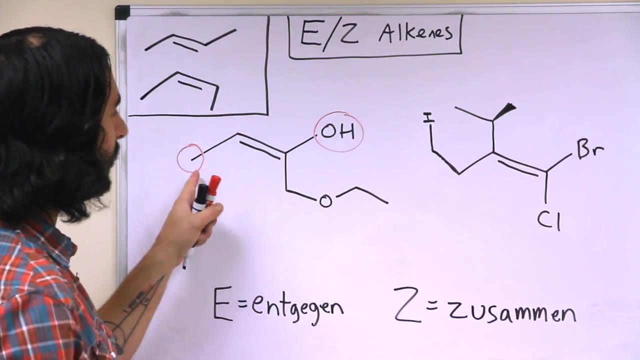 so, actually, this carbon is bound to oxygen and it is bound to carbon, and so this group takes priority, actually because- and for no other reason other than oxygen is heavier than carbon. So we must go one atom at a time. So, once we have determined which two groups take the priority, 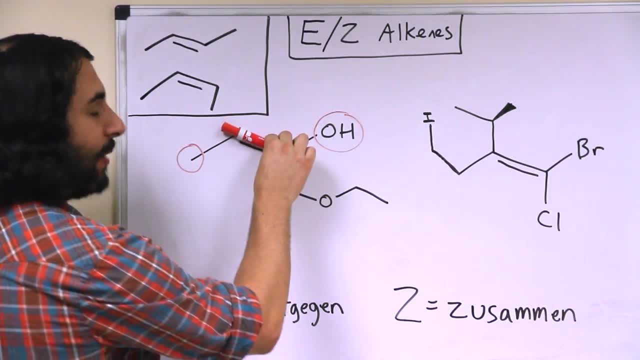 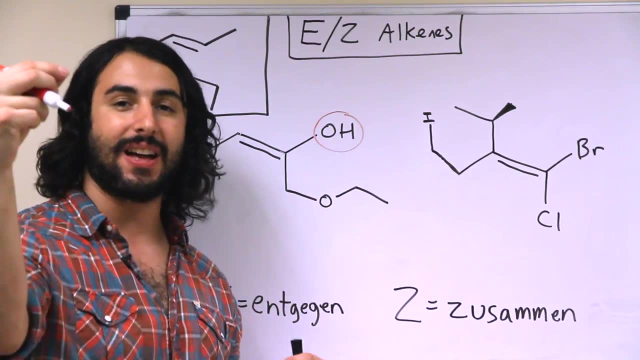 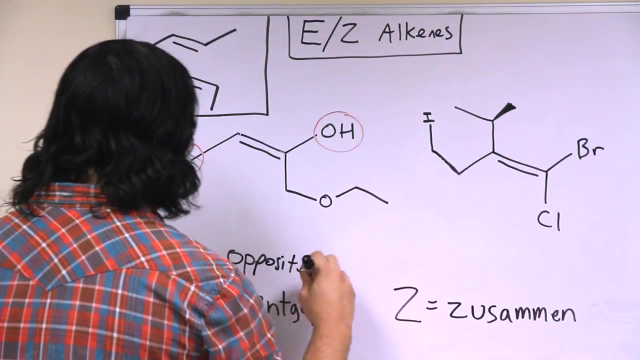 now all we're doing is looking at the plane of the double bond here, and we're seeing that the two groups, the two top priority groups, are on opposite sides of the double bond, And so opposite sides means that this is an E alkene. 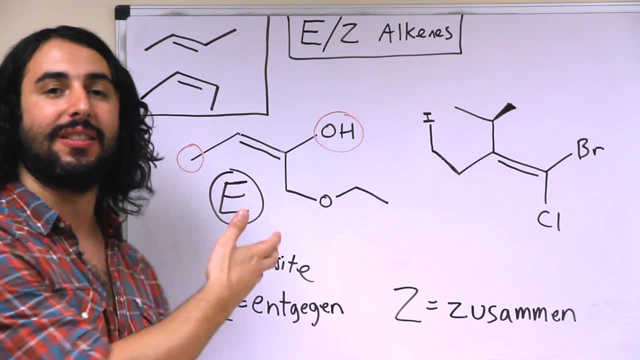 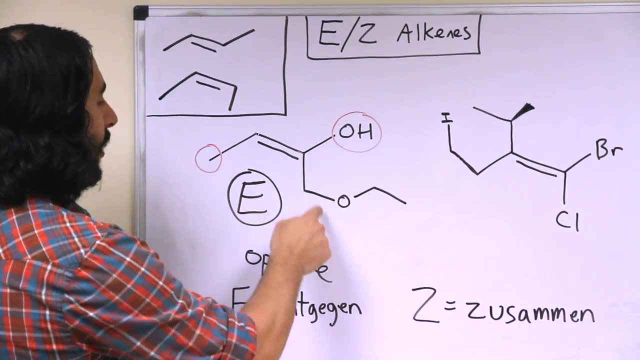 So, whereas for something like this we couldn't use cis and trans, because what would be cis and what would be trans? Well, this group is trans to that, but this group is cis to that, so that becomes ambiguous terminology. but everyone could use the con-engled pre-log convention. 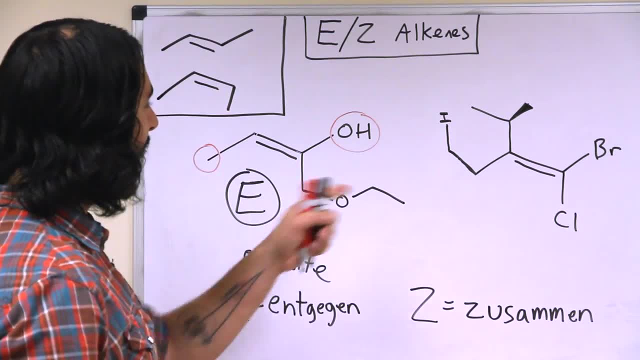 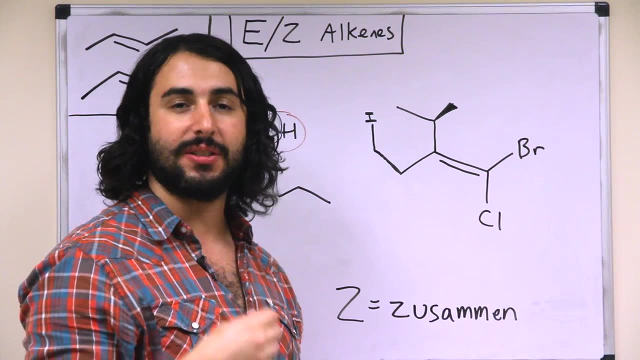 and agree that this is an E alkene. So now let's look over here. So same thing on the right. So here's the two carbons. each one has two groups and we must decide which has priority over the other.